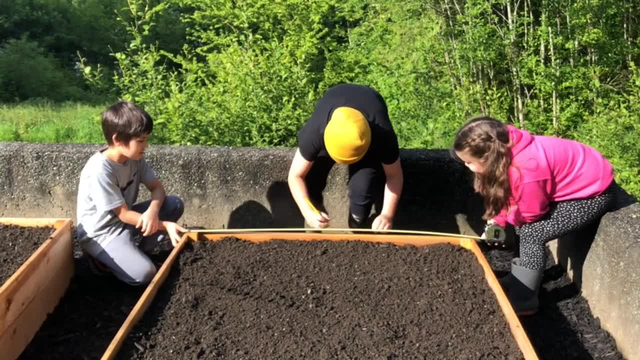 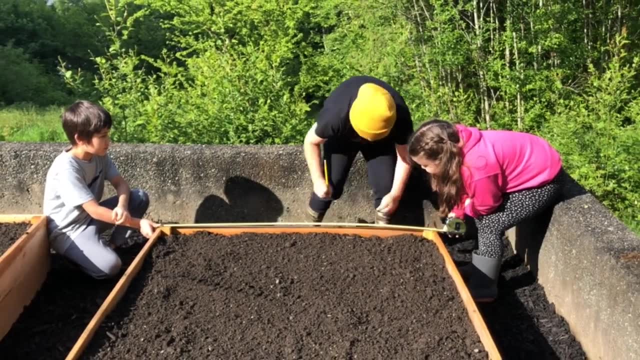 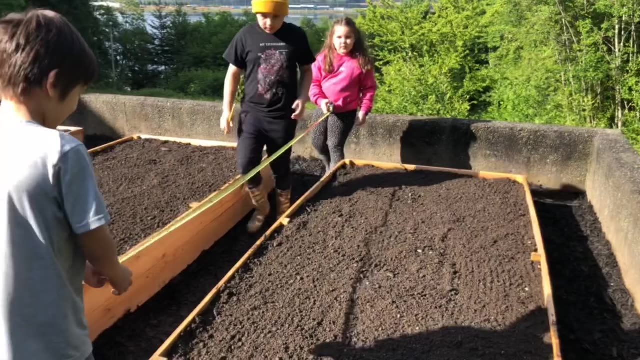 This week we plotted and planted our garden beds. In case you missed the video of us building our beds, we'll put the link in the description, Because we're doing square foot gardening. we had to make our garden into one big grid. We held a tape measure, while one of us marked every 12 inches across each side of the bed. 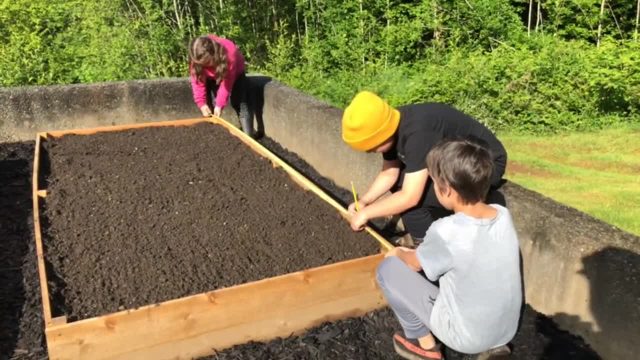 We chose the square foot garden because we wanted to make our garden into one big grid. We chose the square foot garden because we wanted to make our garden into one big grid. We chose to do square foot gardens because they use less water, make the most of the space and allow us to keep track of each seed we plant more easily. 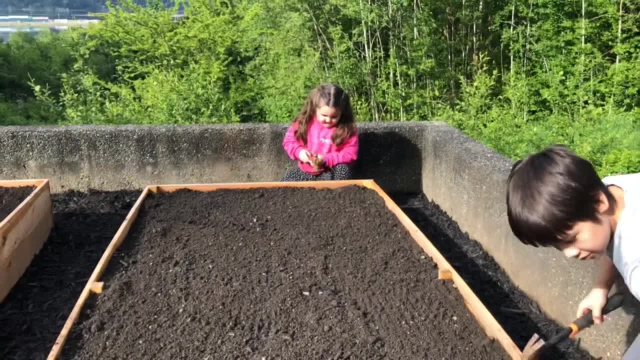 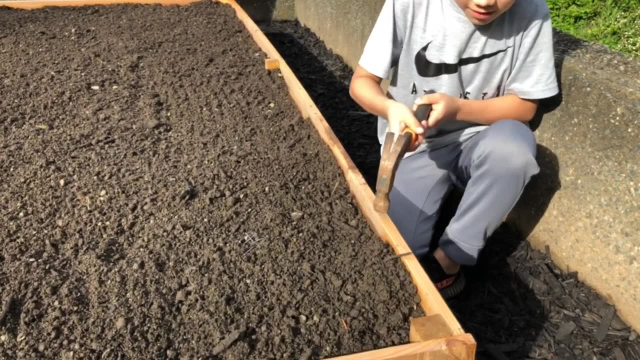 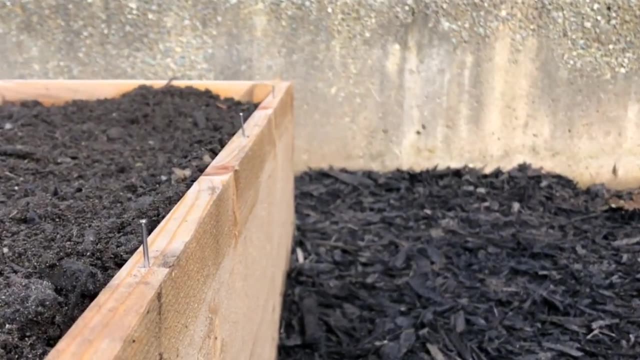 Next, we used a hammer to place small finishing nails in our marks along the boards. We only nailed them in part way, so that we had enough room to tie our string on later. Now it's time to create our grid by tying string around our nails. 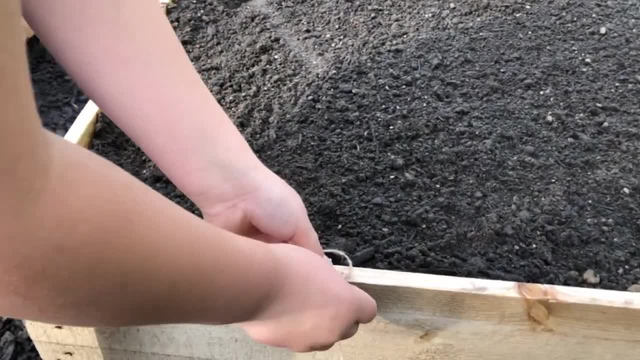 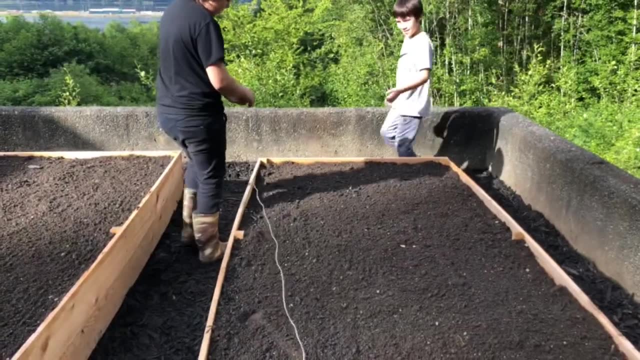 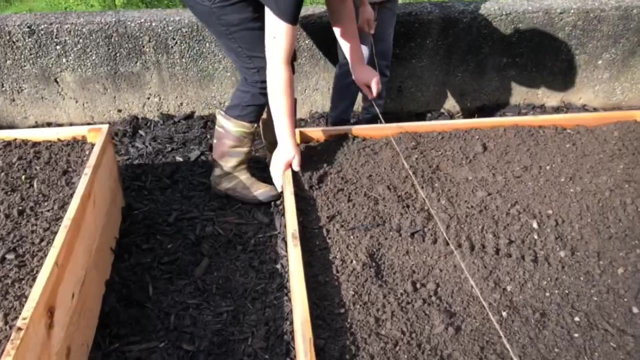 Now it's time to create our grid by tying string around our nails. The trick is to keep the string nice and tight. You can also use wooden joiners to tie the strings around the nails. We will be using a tool called a hook to make the string around the nails. 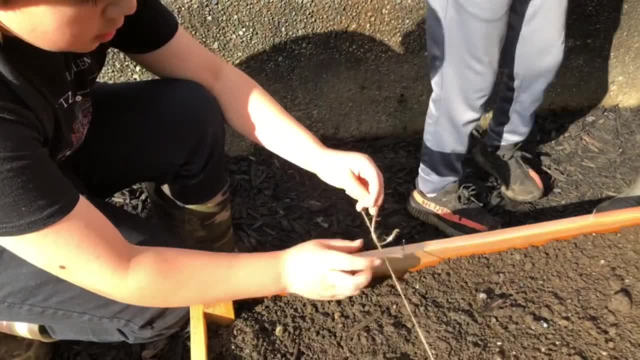 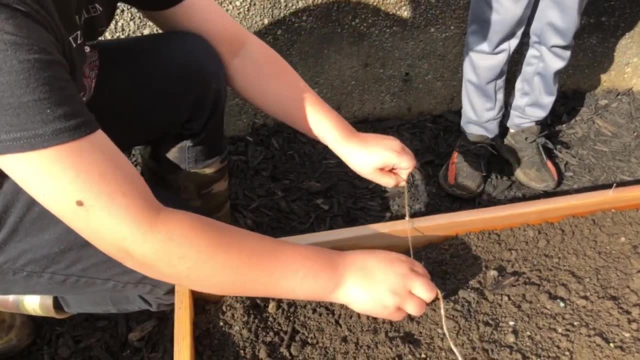 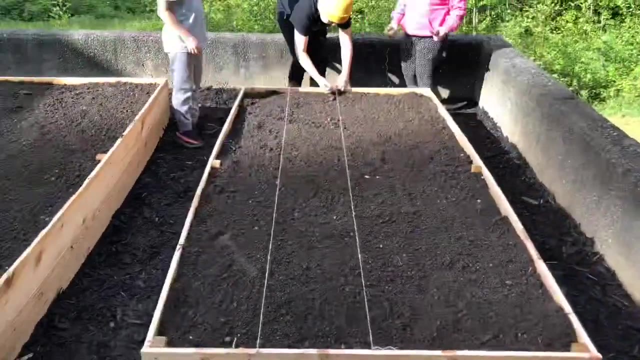 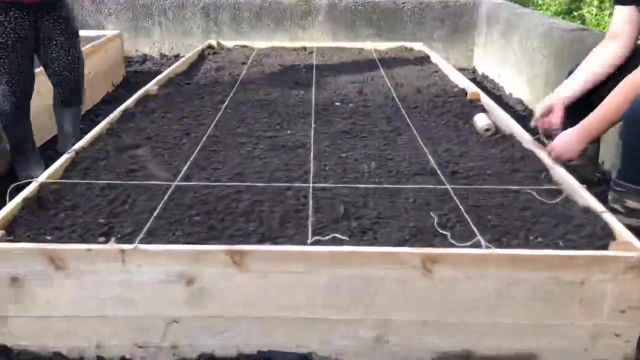 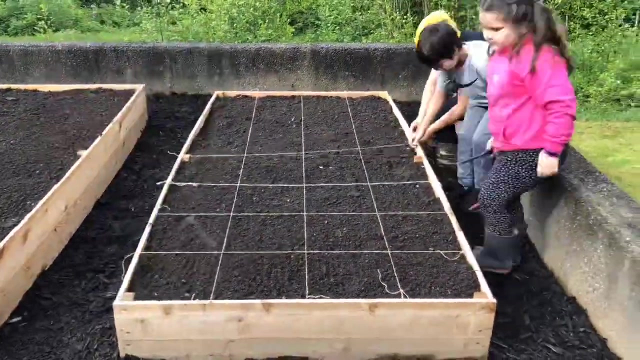 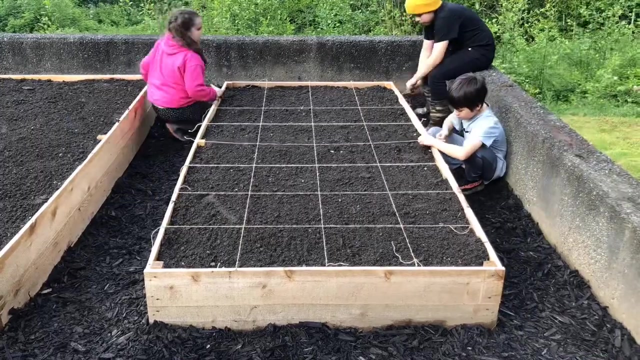 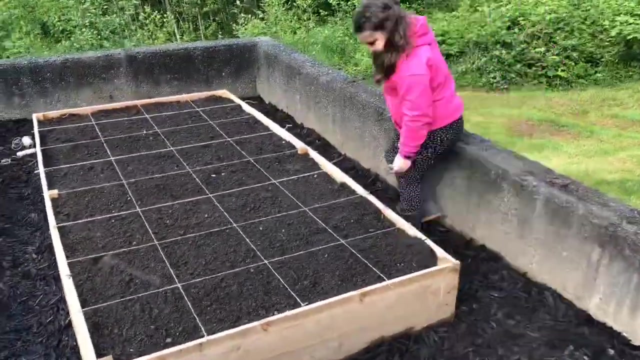 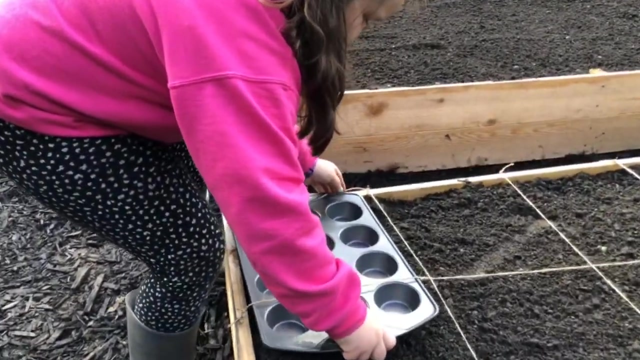 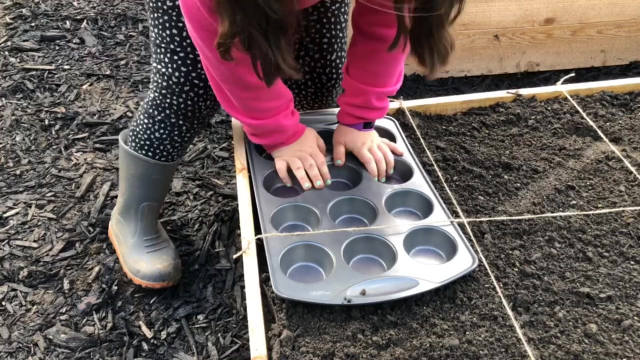 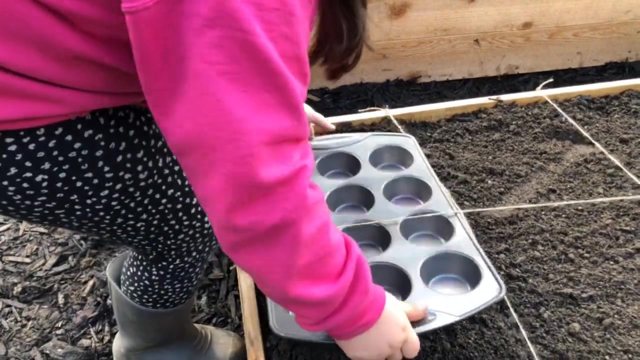 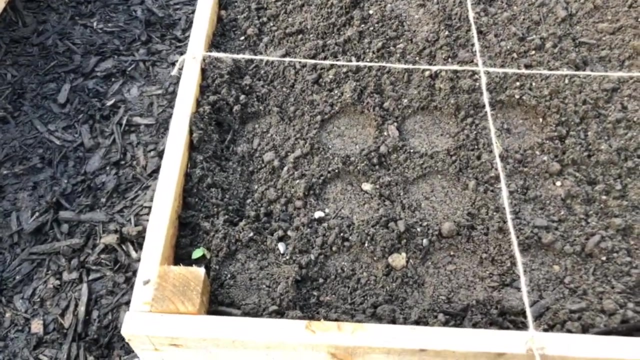 Thank you. By the time this was over, we were basically professional knot tires. Now we're ready to plant our seeds. To make this easier, we used a muffin tin to help us properly space our seeds. Using the back of our seed package, we figured out how many seeds we can plant in each square.